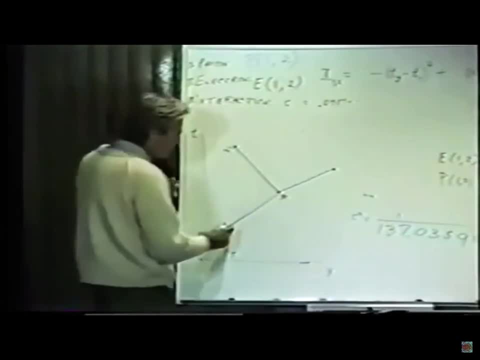 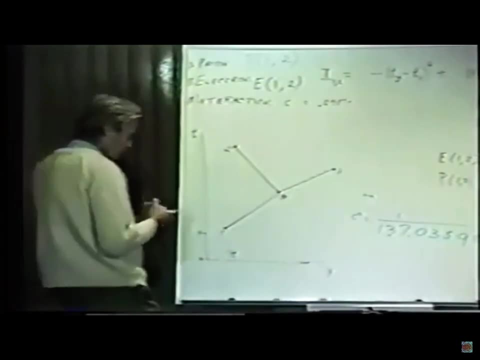 And finally And finally, it arrives at point 2, whereas the photon goes from 4 to point 3.. So this would be the typical amplitude. I would draw a picture like this and I'll tell you how to calculate it. Let's suppose I wanted to calculate the amplitude. 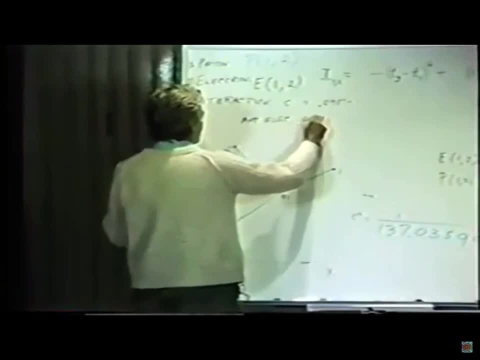 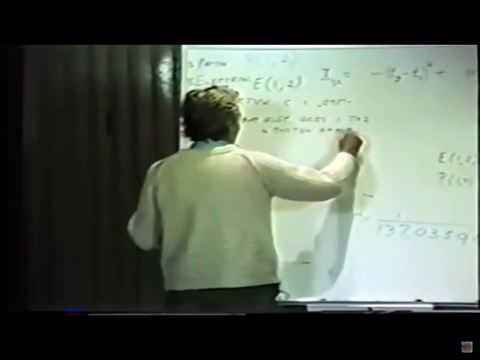 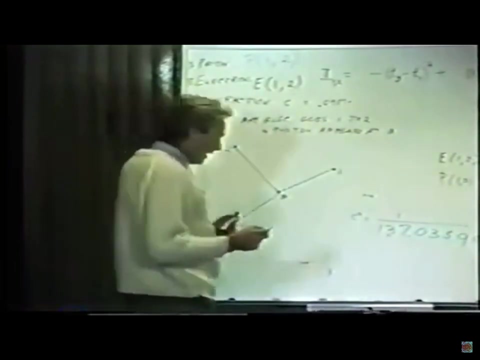 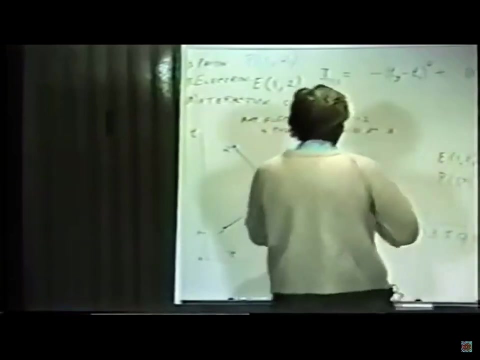 An electron goes 1 to 3,, 1 to 2, and the photon appears at 3.. One way this can happen is one way, only one way, is that it goes this particular way, and I'll call that via 4.. 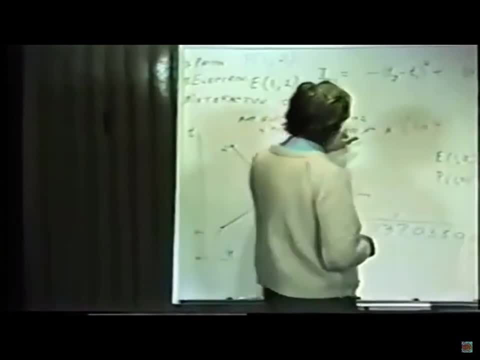 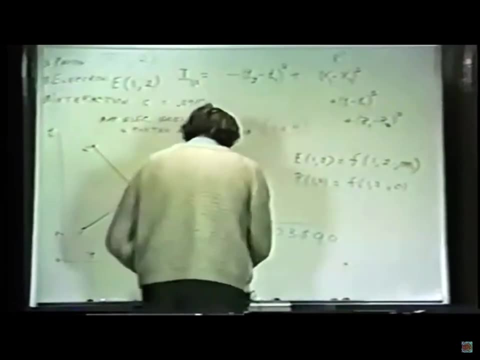 And you'll see what that means in just a minute. It means the electron goes from 1 to 2 via going through point, point 4.. And the photon appears at 3, coming out of 4.. Then the amplitude for this process is the following number: 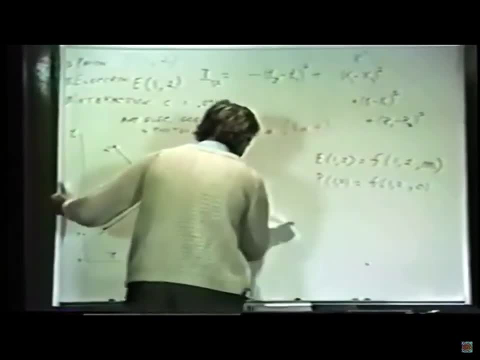 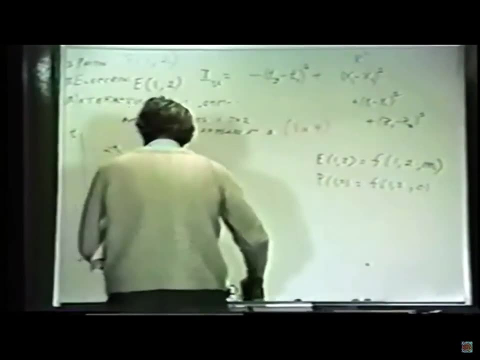 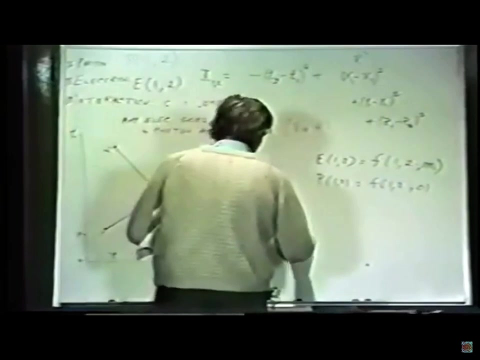 Arrow Arrow. It's the following. I'll write it all down and see if you can understand it. Product: Remember how we multiply arrows. We multiply the arrows. These represent arrows, The arrow corresponding to an electron going from 1 to 4.. 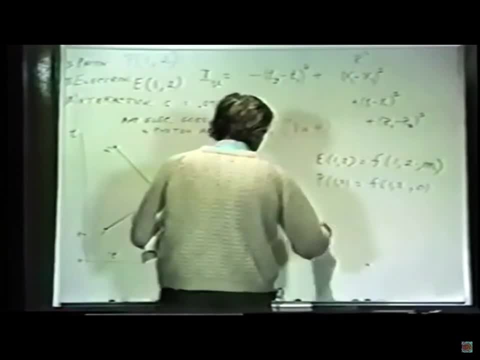 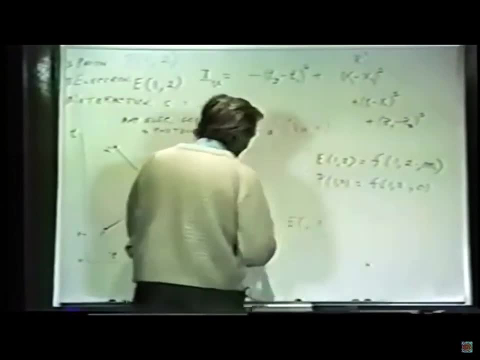 Which, for some reason, I seem to have written these backwards. No, I know, I discovered from experience that to do it the way physicists write it is unnecessary for beginners. It's only a convention. So let's do it the way it looks, common sense. 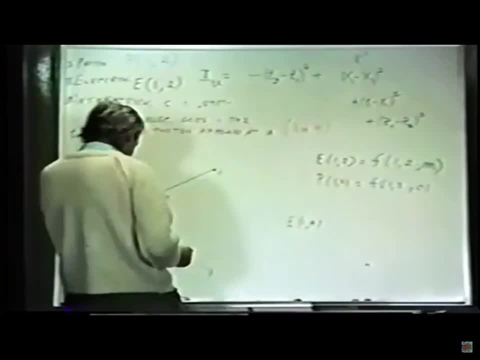 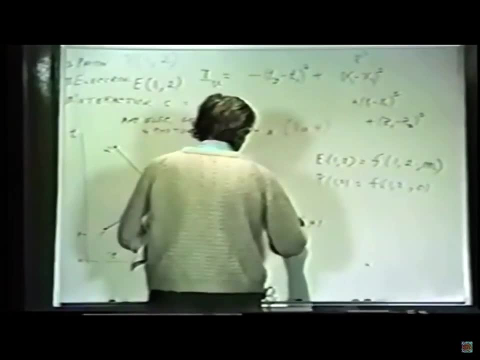 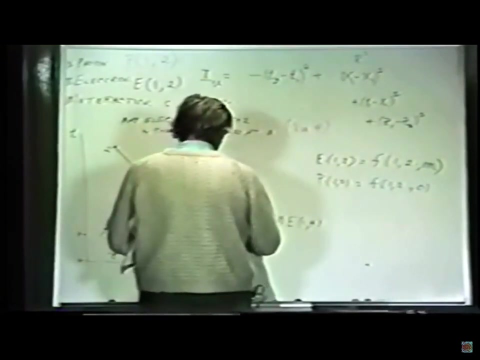 We go from 1 to 4. Then the electron goes from 4 to 2. And the photon goes to 2.. From 4 to 2. There 4 to 3.. Okay, And there was an interaction. 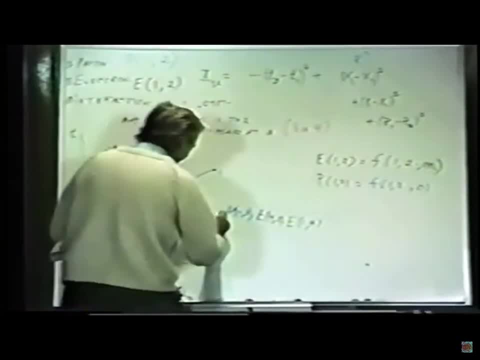 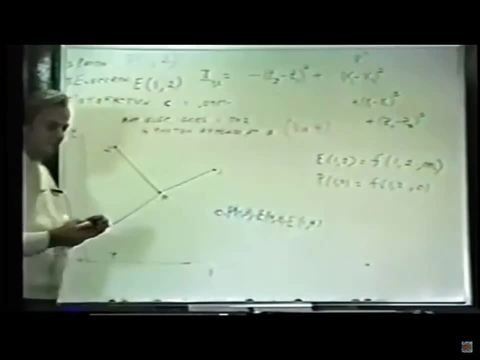 Let's make this nice thing always happen in red. And then we multiply these together, But the rule for multiplication was explained before. They rotate and shrink. So you figure out what each one of these arrows is And rotate and shrink. So this is nothing but a shrink. 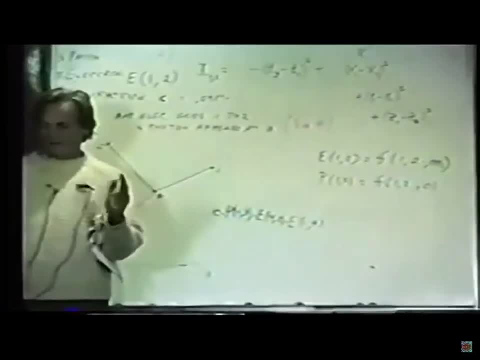 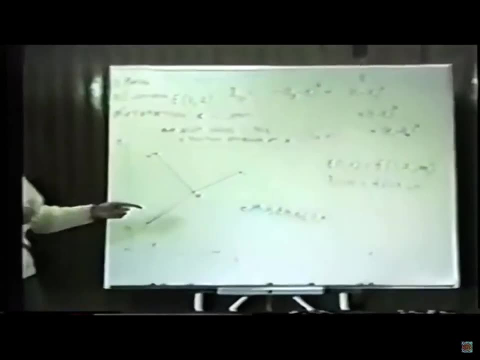 It always says: If you have an interaction, shrink the amplitude by this factor 0.098,. whatever it is, I don't remember the number. Okay, I can remember the square upside down, but I can't remember the square root. 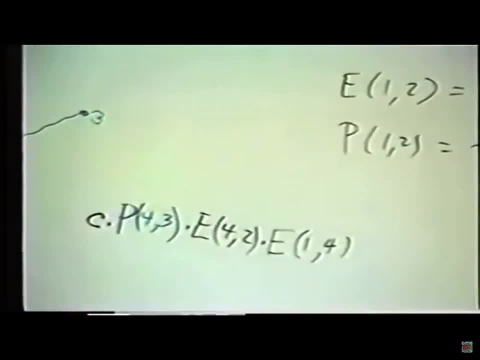 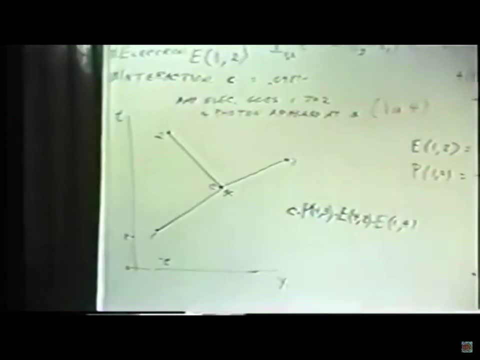 So whenever a photon comes out or in, like this, and you draw this, that's where the C appears, The shrinking Each time you emit or absorb a photon, And the motion of electrons going from place to place is always governed by this. 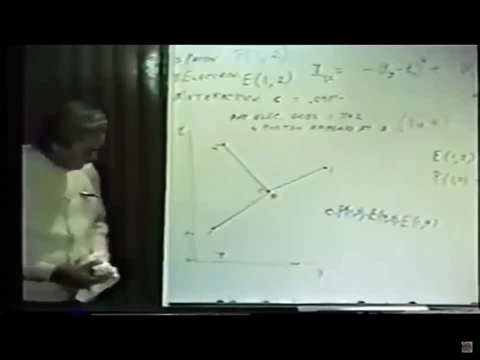 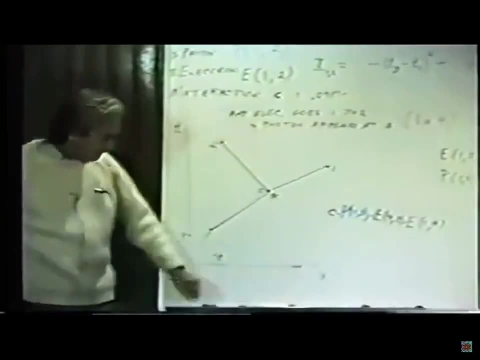 and the photon, always by that And by that way. in that way you can figure out the amplitude for anything, Because a whole world of electrons and photons, at least, is nothing but these three processes combined in various ways. That's all. 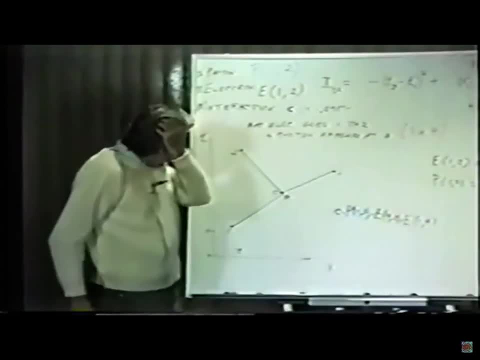 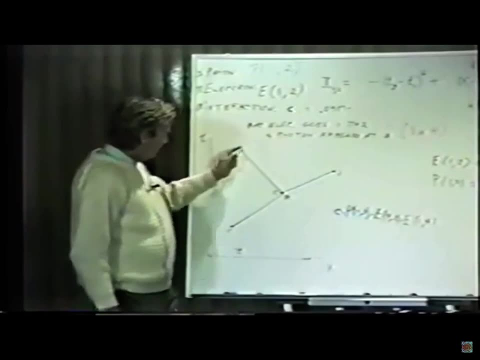 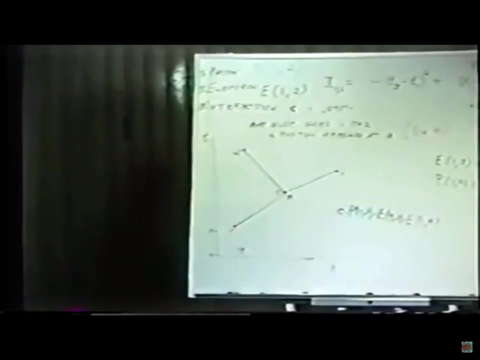 It's done. Uh, One point, however: If all I knew was that the electron started here and ended here and the photon ended here, this isn't the right amplitude. Why And what would you do to do it right? Huh? 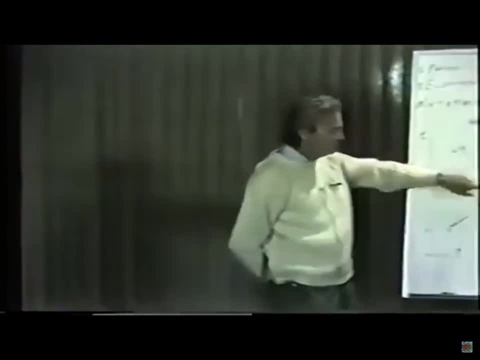 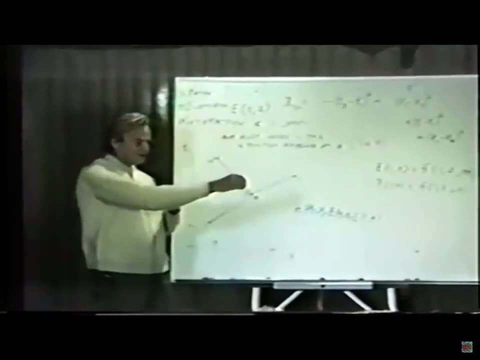 What? Yes, You don't know where 4 was. This is the hour if it happened to do it there, But it may have been that number 4 somewhere else It might have been. this point is here or here, or here or here. 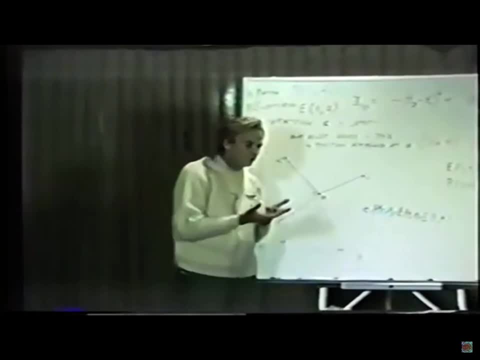 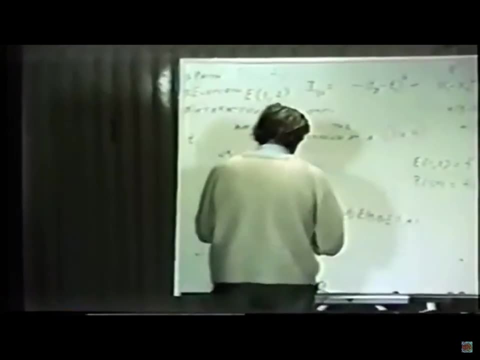 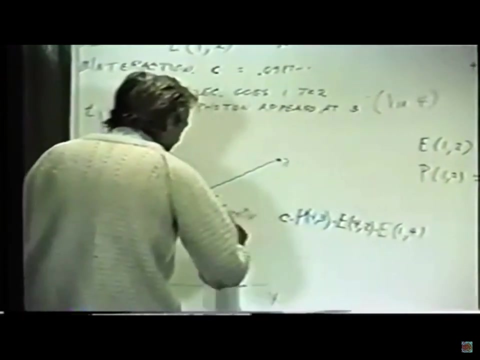 And for each of those points there's a total amplitude. Those are alternative possibilities. Those amplitudes have to be something, They have to be summed. So we could say We have to finish this for this particular problem by saying sum on all possible places. 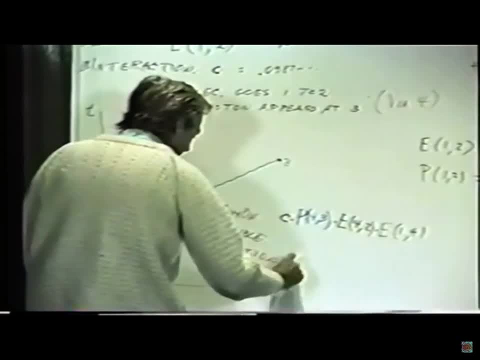 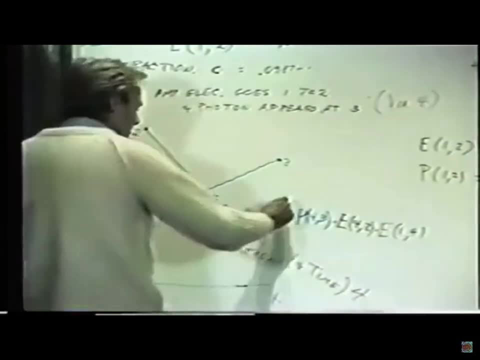 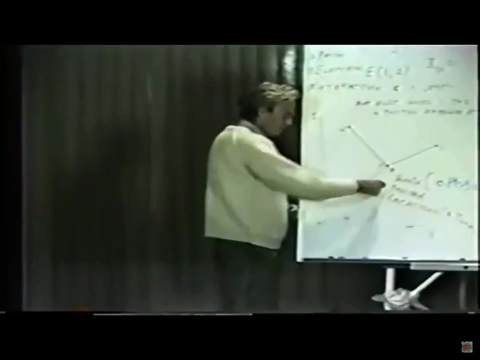 locations and times that I've labeled 4.. Sum this, Make this arrow for every place and add them all together. The square of this would be the probability- the square of this mess would be the probability- that if an electron were liberated here, 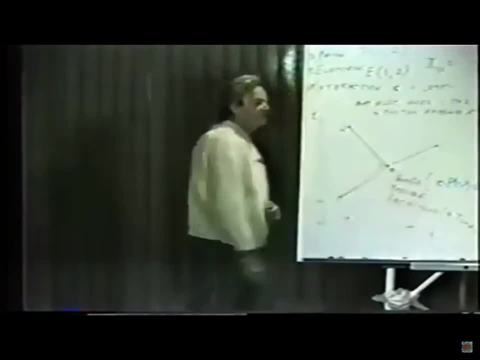 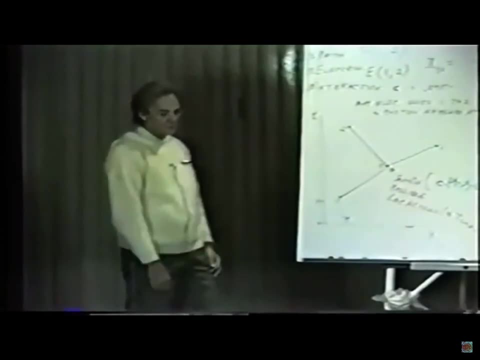 and were found later here, that you'd find a photon in the detector over there at that moment. All right, That's the special problem And that's the answer to it. Almost, I have to tell. there are more, always, more diagrams, more pictures. 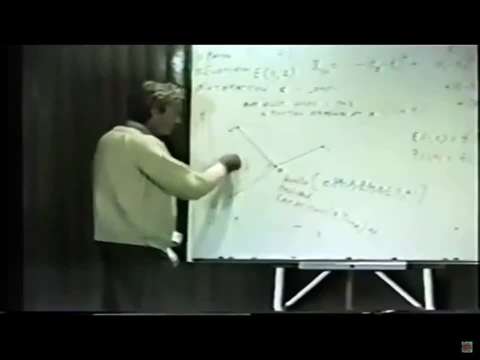 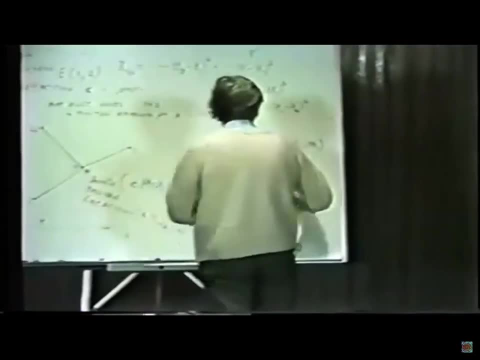 more ways, Because this electron might have emitted a photon which was later absorbed by the same electron later, and all kinds of terrible things Which I now will explain. So let's take another problem. Well, this is a good one, but we'll leave it there. 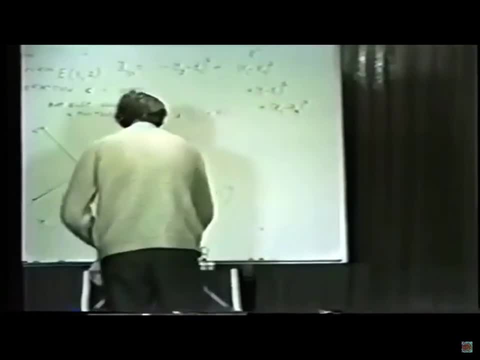 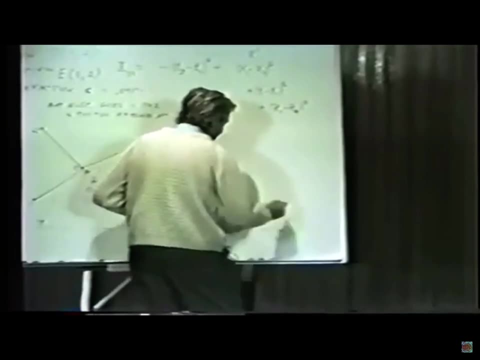 But we can take other ones to show how it's done. Suppose that I talk about what's called usually called the scattering of two electrons: One starts at a certain moment from some place and another starts from a moment from another place. 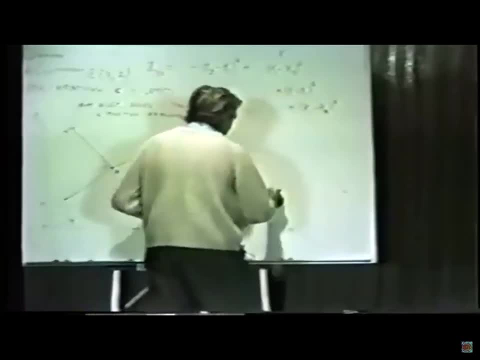 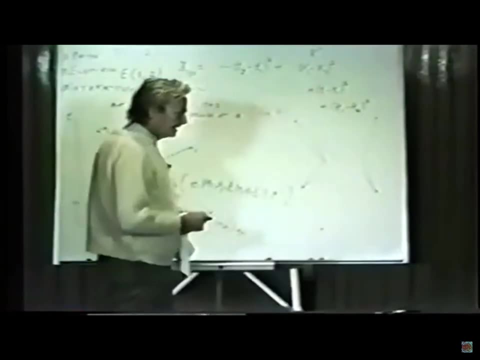 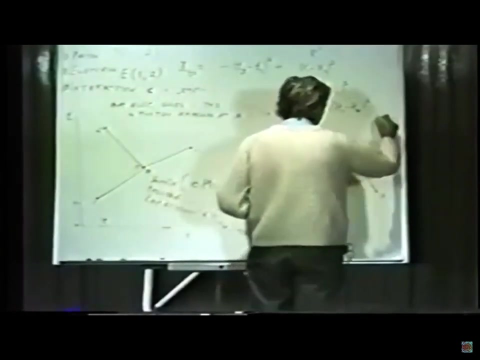 and later you find them in two other places And therefore we have an electron that may have got from here to here and the other one may have got from here to here. Now let's calculate the amplitude for that. Let me call these positions 1,, 2,, 3,, 4.. 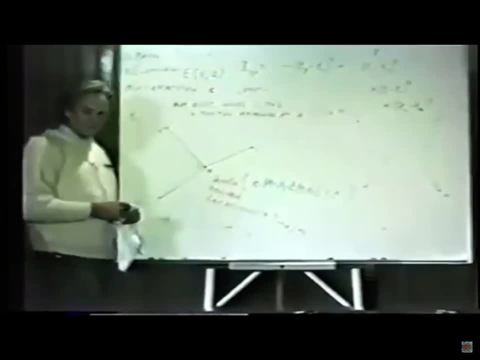 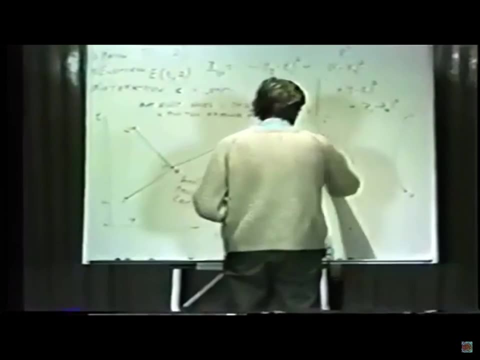 And I'm going to make a little, a few mistakes. I'm going to rush fast and you're going to have a few mistakes. we'll come back and fix. First of all, for this problem, I'm drawing this line to save the other thing for the blackboard. 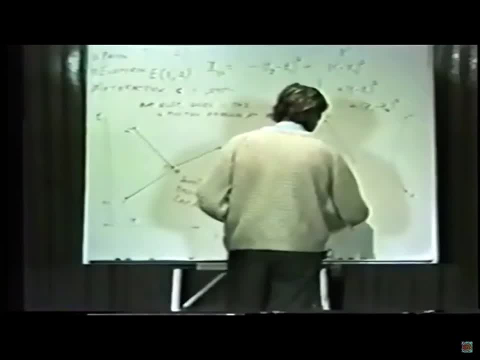 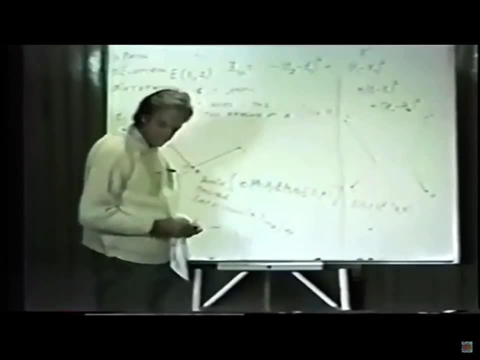 For this problem. the answer is simply E21, E12 times E34.. All right, Electron went from 1 to 2, electron went from 3 to 4.. Okay, Anything else. Any remarks Finished? Not quite. 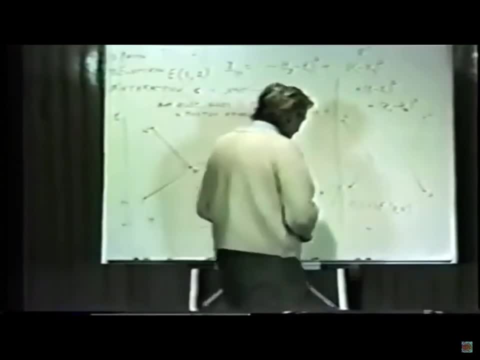 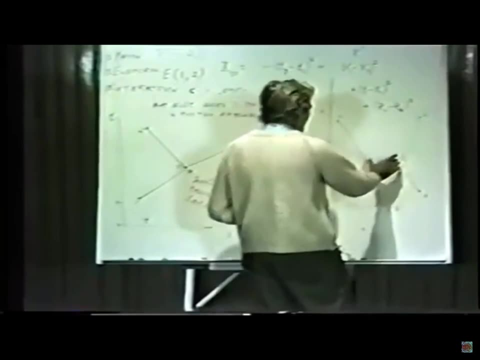 The photon went from 1 to 4.. Yes, a photon can go- Not from 1 to 4,, but you could have a situation like this. This is the first picture. I haven't got room on a blackboard. I'd just love to keep this one. 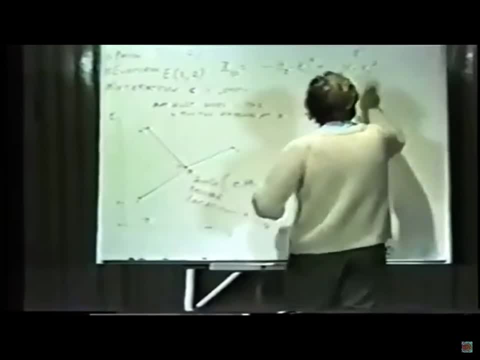 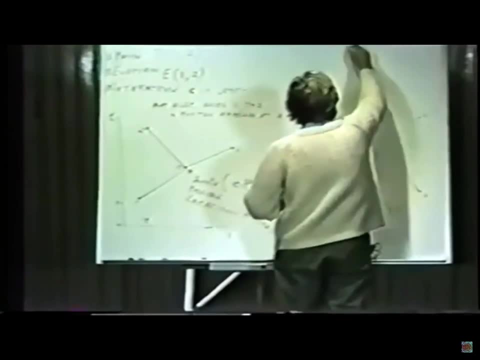 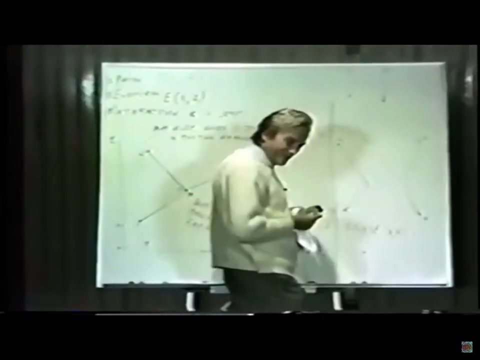 Well, let me erase this and make the picture smaller. So this first picture is now redrawn. Here's 1 and 2. And the second picture, 3 and 4.. Now, this is now going to be the basis for the second picture, The second. 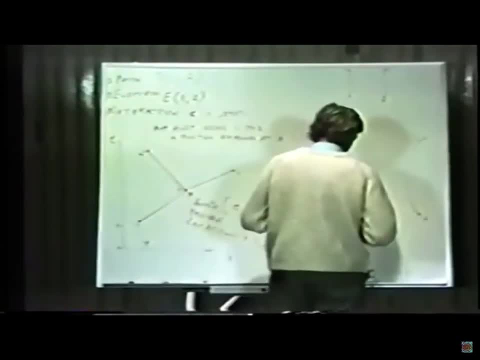 picture has a new possibility in it. That is, that the electron went from 1 to 4 or 5 and emitted a photon, and the other electron went from 5 to 6 and picked it up. Yes, and what we're asking for now is the amplitude- a new problem. that's part. 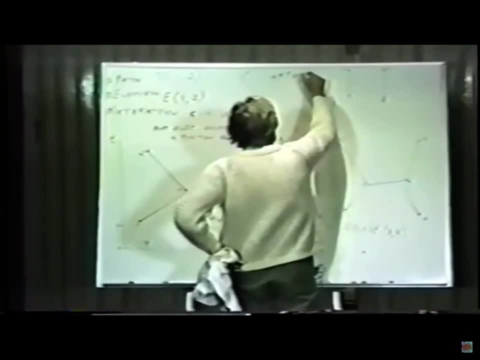 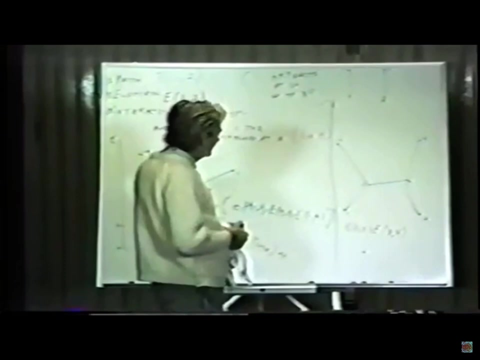 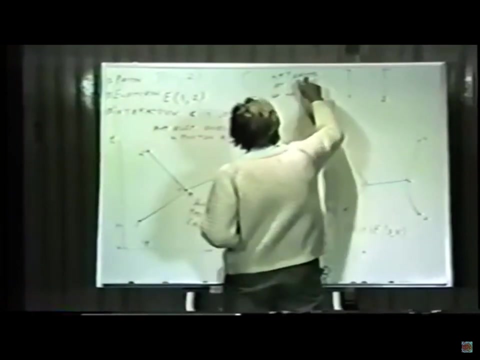 of this section. amplitude of electron, originally at. electrons at 1 and 2 go to 3 and 4.. All right, What's wrong? Of course, you're absolutely right. Electron 1 and 1 and 3 go respectively to 2 and 4.. 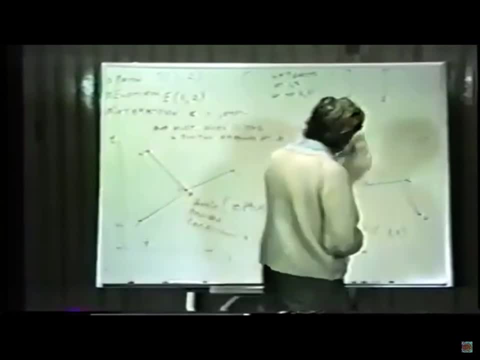 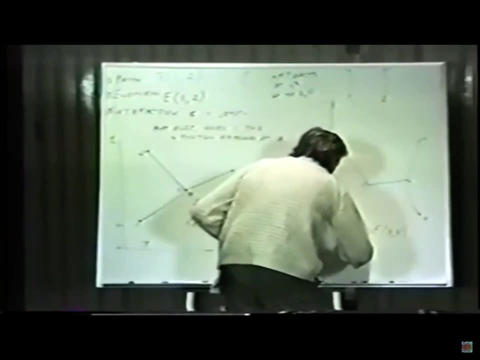 Okay, Now, this was the first term That corresponds to this possibility, but this is also a possibility And for this possibility I'll write it down. I'm not going to write any more because you'll see very quickly what that is. You're learning the principle. You're not going to actually 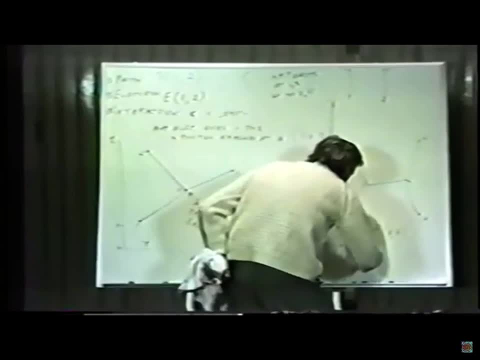 calculate because we don't know the formulas, But this would be things like E51.. This would be E51.. This would be E51.. This was times you remember in the normal business of time Times: E25, times, E63.. How? 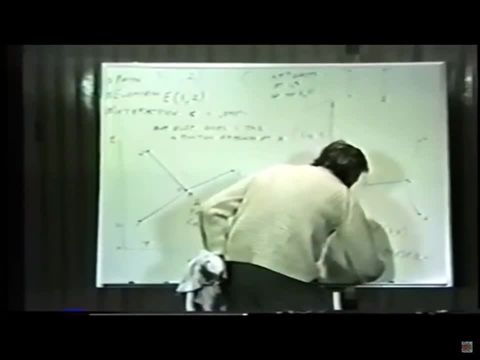 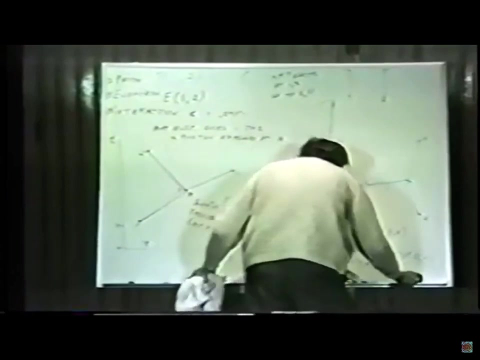 brainy do you have to be to write this down? huh, 46 times. ah, wait, a minute, now got to get a blue one. Yes, you do, Yes, you do. Times P56 times more, Yes, more, More Yes. 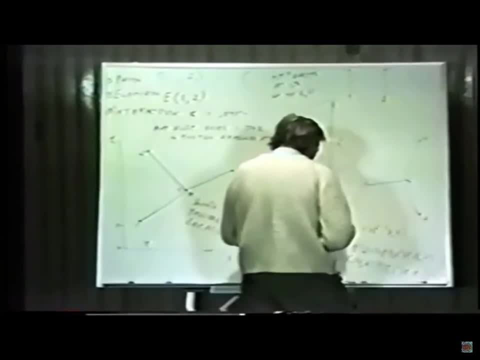 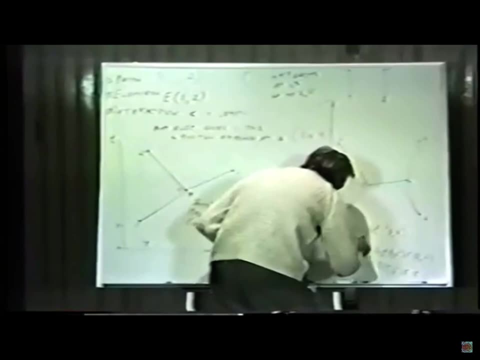 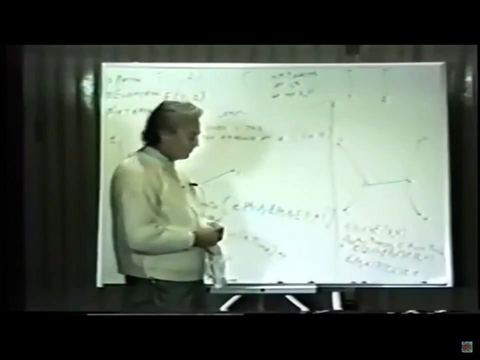 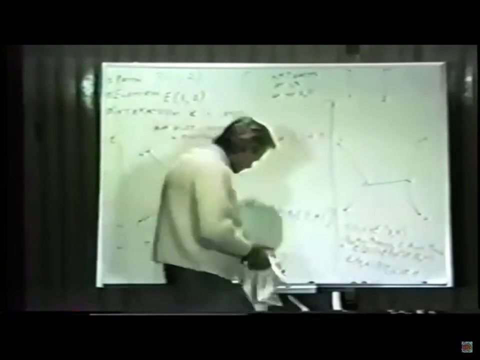 more Times. C, Anything else. Oh, yes, Sum all places for 5 and for 6.. Okay, Well, you get the principle. now You have all these things happening. You multiply the amplitudes for all the things that are happening. What are those C's? Those are the junctions for each. 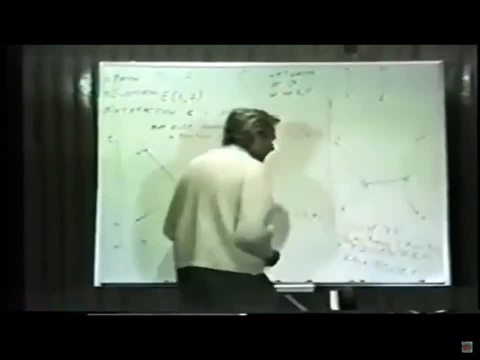 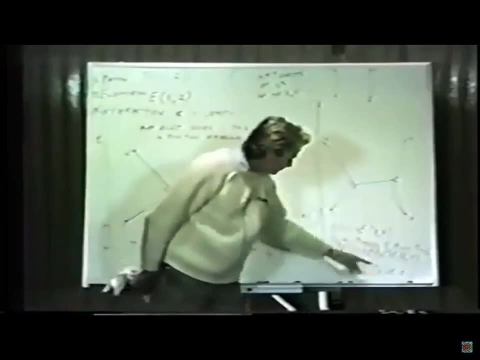 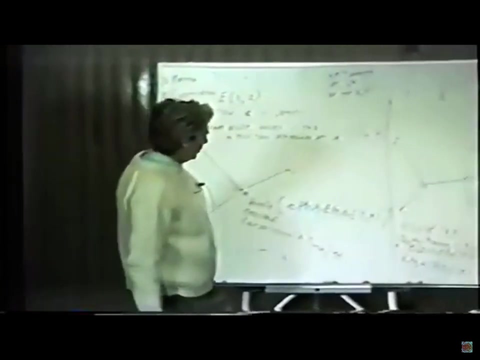 junction for each interaction, We have a factor C or an amplitude C, a shrinker, And all of these are the amplitudes for the things to do what they have to do. Now I have some questions for you. One: what about the possibility that this photon simply comes out here instead?